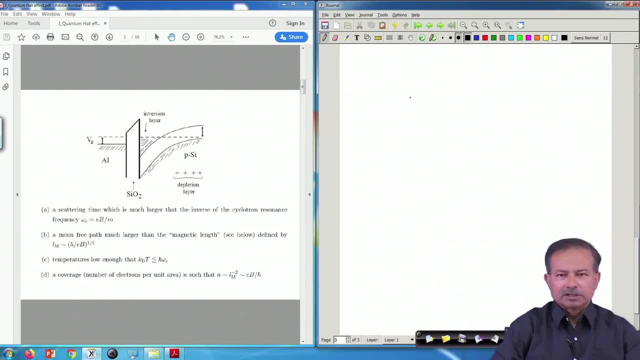 so that they become two dimension. the carriers become two dimensional carriers in. they move in only in two dimensional. So let us me show you how it is done. So the geometry of this device is this. that let me draw it, ok. 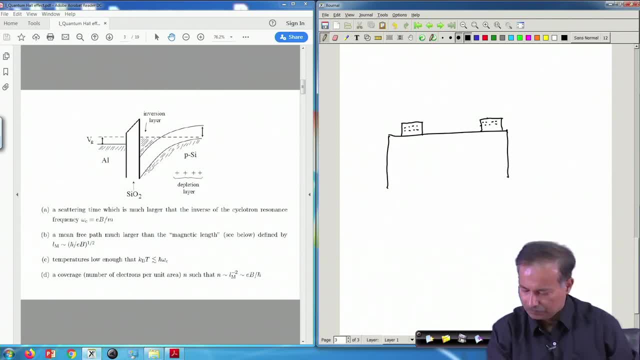 So let us see, Ok. Ok, This is a MOSFET geometry, MOSFET configuration, and there is a source and there is a drain here- sorry The- and there is a silicon dioxide layer, Si O 2. these are also Si O 2. these region are. 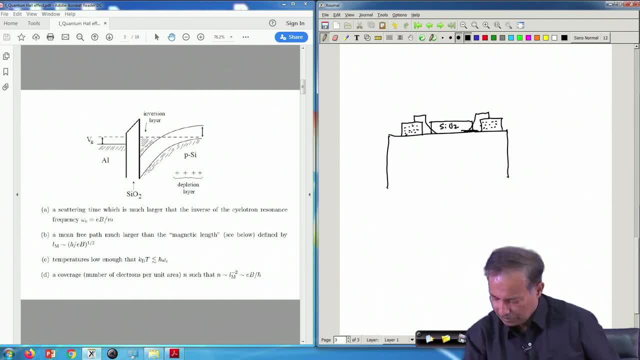 also Si O 2.. Ok, Ok, Right, Ok, Right, Ok, Ok, Ok, Ok, Ok, So that you can see this: It will create only one component, another component also, there is another component". then you have this source and drain. these are the source. 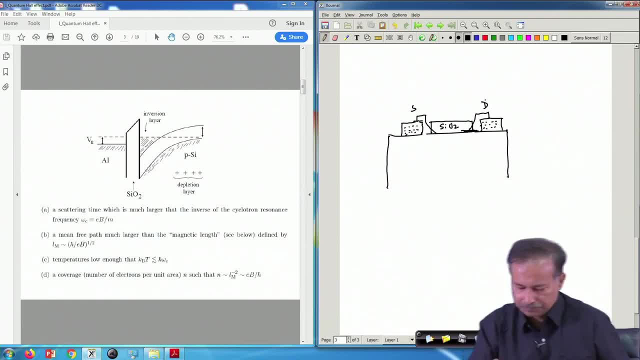 and drain. These regions are source and drain, And so what you do is that you apply a Ok Here, and then on top of this you put a aluminum, metallic aluminum, and you- this is this- acts as the gate. So this is the V gate that you apply here. ok, 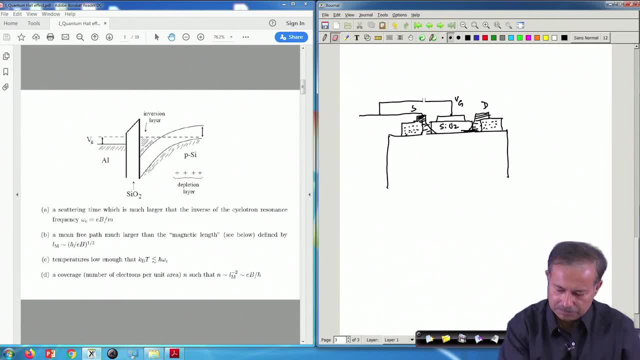 So this is in this case, this is kg. is respect to this? ok? So this is the configuration. from here on drains out. So this is the typical and this is p type silicon: ah. So because of this configuration, you will have a. 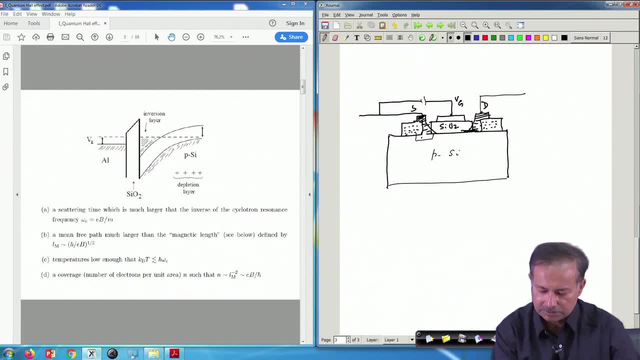 n plus layer here, n plus region here, and there is a confinement of electrons of the carriers in this region just below this SiO 2 layer, and they are confined. I will show you why and how they are confined. So the axis is such that the downside is: 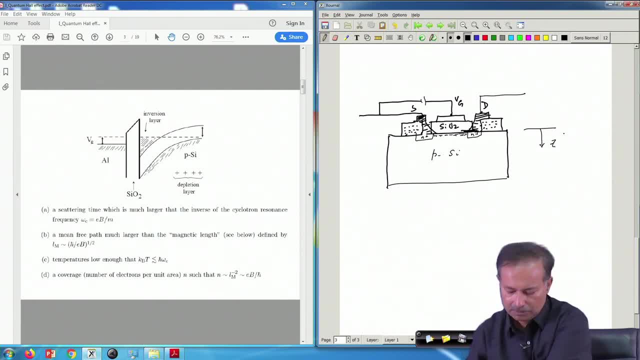 z. So this is my aluminium gate, If I draw the energy diagrams in this system. So let us, Let us just draw it. this is my aluminium gate. this is the SiO 2 layer, and then there is a region And it is called inversion region, and there is a depletion region z d, which is like this: 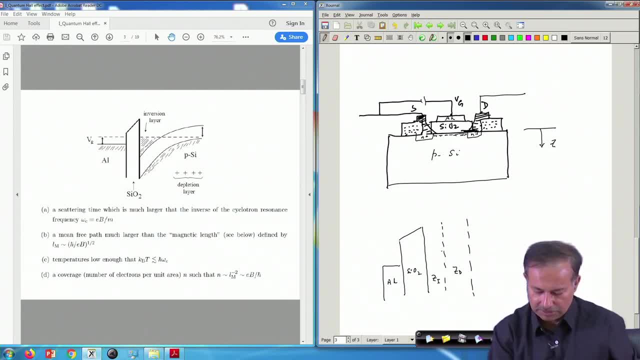 and what you are doing, is that? ok, Let me just plot first, and then I will show you what I mean. ok, So I have this valence band bends. So I have this valence band bends. So I have this valence band bends and the conduction band, which is like this: and this is where 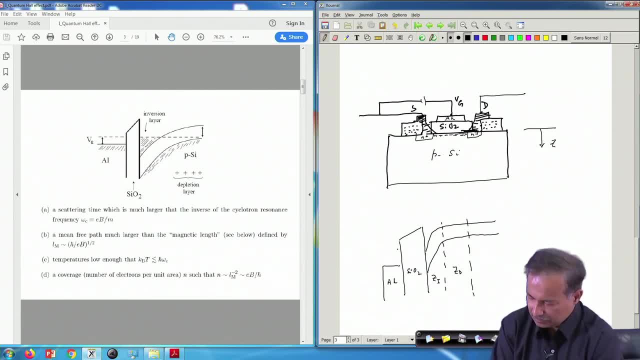 the E f is ok, So this is somewhere the Fermi energy is. Now you put the gate voltage, So this is where the E g at, here in this, here at the aluminium, So that you can now move this Fermi level up and down. or other way to think about it is, you can move this conduction. 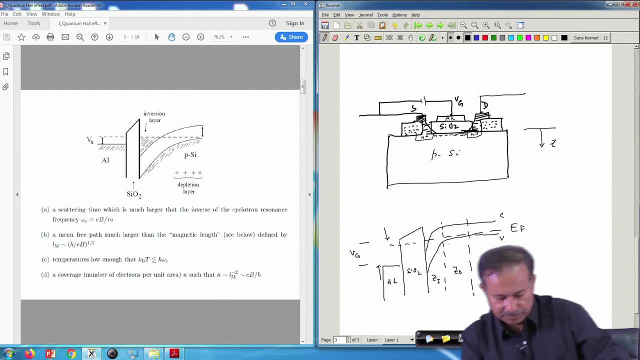 and valence bands up and down. The better way to look at it is that the we move the Fermi level up and down. by doing this. Now the valence band, since the since this, this region of the conduction band has come below the Fermi level and it is a region of 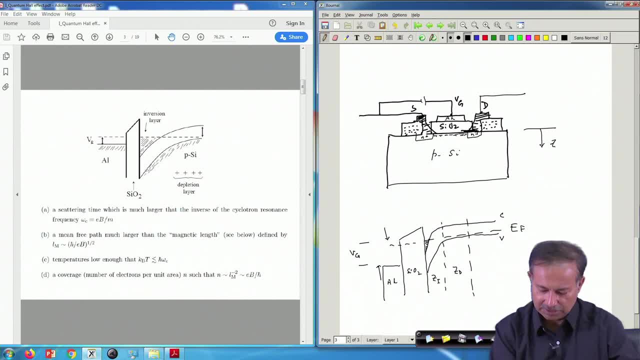 and the potential. So why does the potential look like this? Earlier the before I applied a gate voltage, The potentials were straight horizontal lines. this, C and V were horizontal lines, whereas now what has happened is that minus because of the electric field coming from the gate. 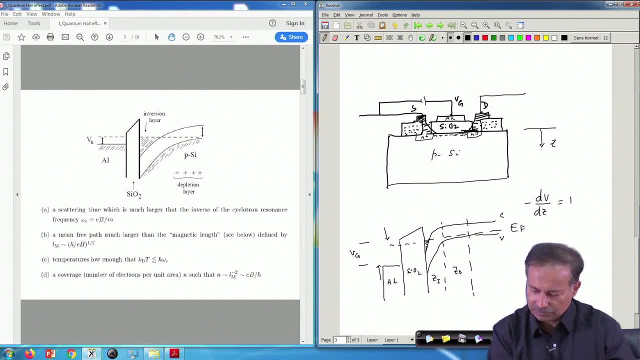 you can, you have to solve this equation. this is equal to your electric field. So there is a field inside that field bends these bands And so the bending happens because this electric field is constant and your V then is V equal to 0, to z. See, at 0 the value is the same as V, g, then E times d z. ok, So this is the 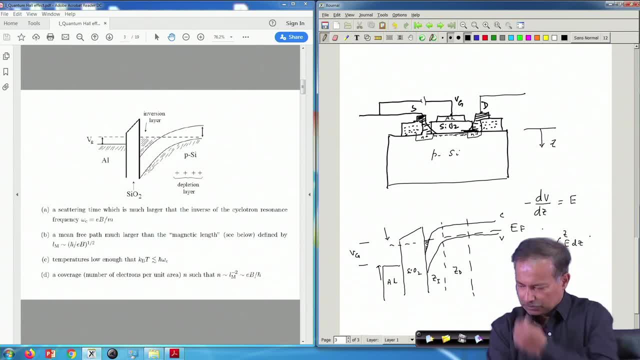 eta term Cel ones equal to del to V c. So what you get is a, E, V, E, v, E c then goes to E c minus E times V, g minus z, e, And E v goes to E? v minus E times V minus G, e, and. E, g plus C, l, z. I have done that many times Here. let me stop. Let me, when I add them together, I need to write them strictly. Let me turn off all thecej andWait a minute, I'll not finish them all. Let me substitute all thec, but these are an vitamin C and vitamin. 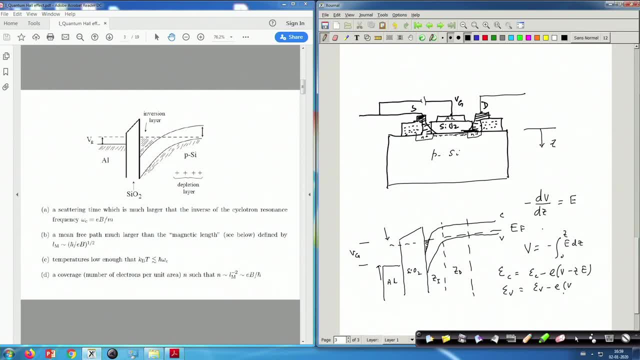 six, There are some antiseptic compounds. Please see what it is and visit at Sherlock College. v means v g. at 0 it is v g minus z e. So that is. that means there is a proportional to z change. So the whatever potential was there, suppose this was the potential. and now 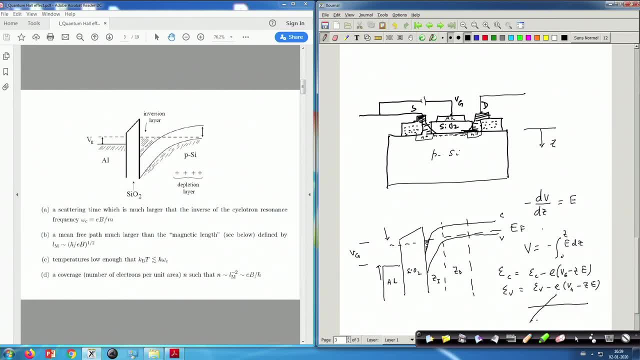 you apply another one which is like this: So the net effect is a potential like this: ok, So that is the way the bands are bent, and then the electrons get transferred from here to here, and these are. these are the electrons which remain confined within this distance. 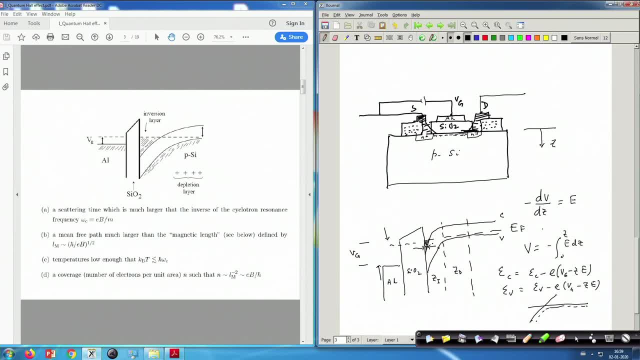 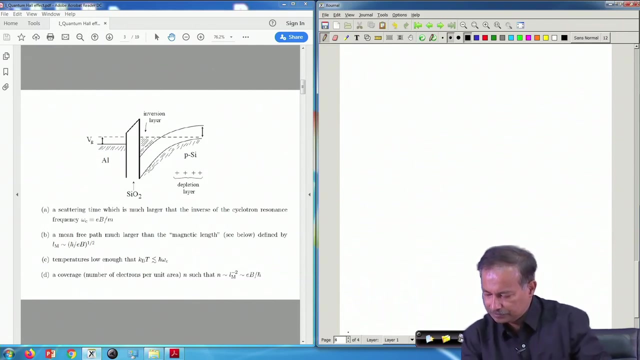 ok, So that confinement is what has to be achieved within few nanometers or so, depending on the other parameters of the system. So that is how the confinement works. ok, So once the confinement is achieved, the rest is basically very simple. we have to solve something called a Landau problem, So these: 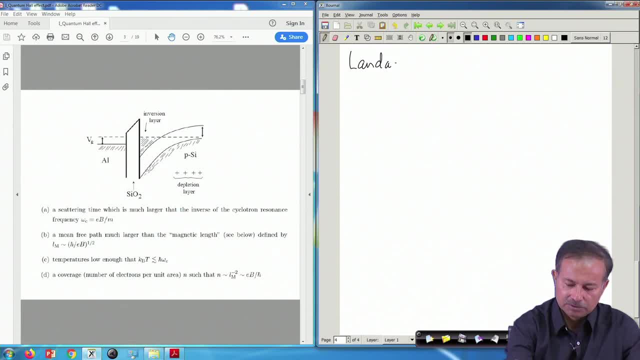 are called Landau problems, So these are called Landau levels and it is basically 2 D electron gas. So that means the it is confined in one direction, which is z here for us electron gas in a strong magnetic field. 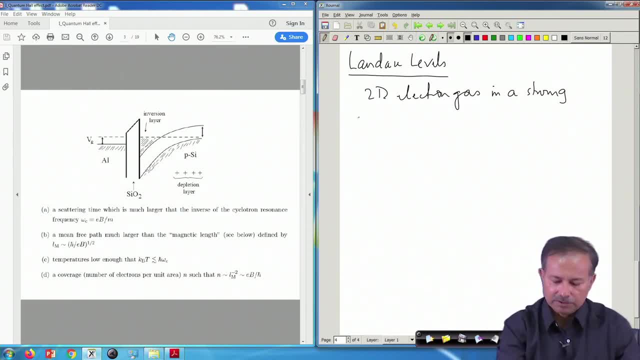 So this is required for the experiment. but Landau problem, you can do it any magnetic field. So that is the problem that one needs to solve now. ok, The way to do it is that. see, the other thing that one assumes is that the spin degree of freedom is already frozen because the magnetic 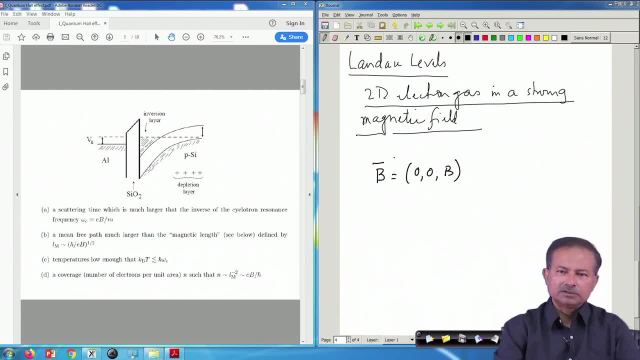 field is fairly high. So the spins have all aligned along the direction of the magnetic field. So we will not bother about the spin part of the Hamiltonian. that will not give us any new result. So then the only the orbital part is necessary. So P, we know, under magnetic field goes to: 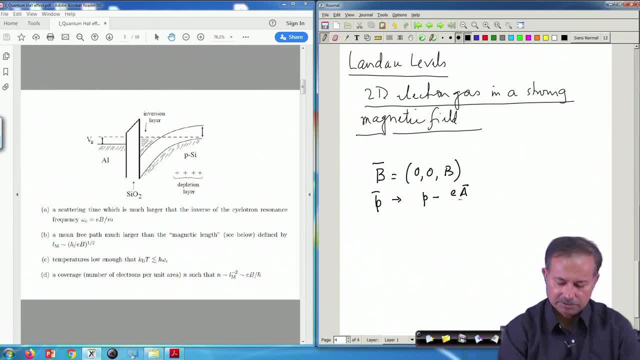 P minus E, A by C, right, So E here is of course negative, and the other thing that we have to use is B, where B is equal to curl of A. ok, So this is the vector potential that we have all done in our electrodynamics, and P minus E A by C is the canonical momentum in presence. 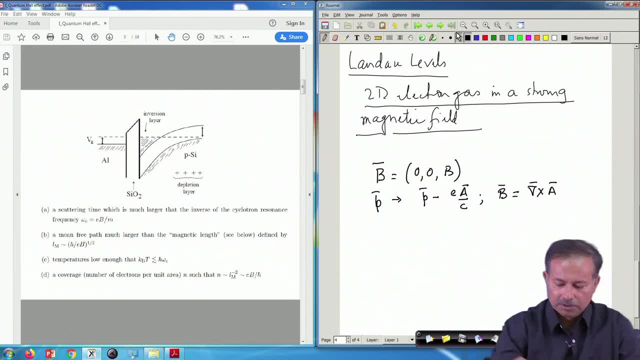 of a magnetic field. So in this we have to just incorporate into our theory. So for that we need to know what A is A of course has we remember that your electrodynamics, you can have a choice of E. 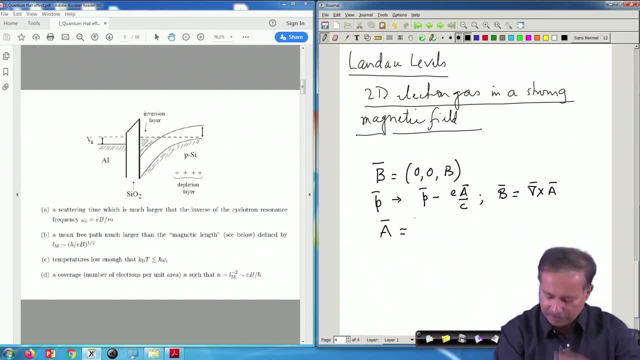 Which is, you can choose in several ways. there is a freedom of gauge choice, So one choice, which is convey, is So A. you can choose as minus y B 0, 0, or you can choose in another way: 0 x times B 0.. 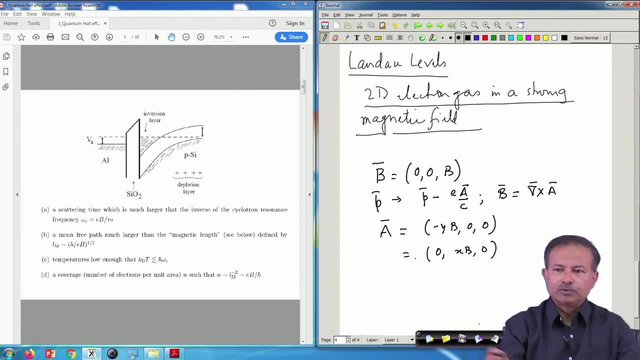 So both the choices are perfectly all right. this is called the Landau gauge. There is another way you can also do is something called a symmetric gauge, which you can choose as a combination of both, keeping both of them for your A. 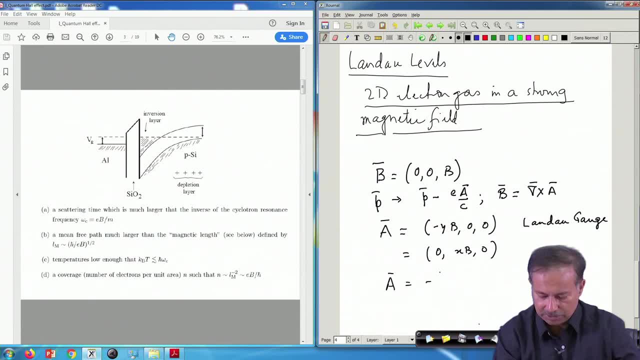 So symmetric gauge, for example, is minus half, minus y, B, x B, 0.. So this is y times B, y times B, x times B and 0, of course. So this is called the symmetric gauge. You can work in any gauge you like. 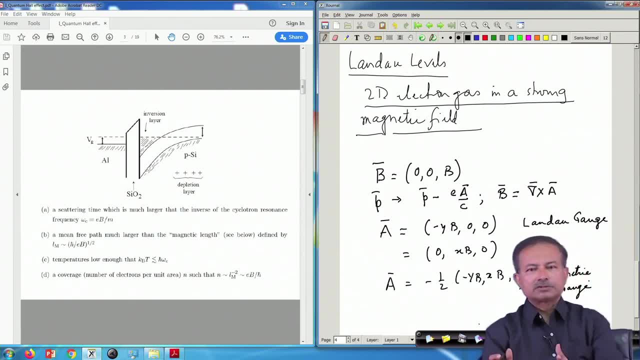 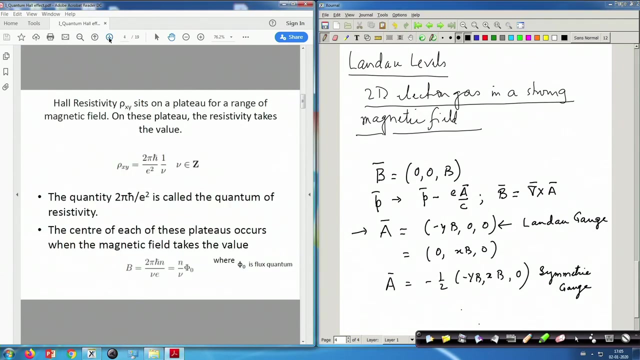 And different books of different notes. you will find work in different gauges and we will not discuss much of it. We will choose one particular gauge, which is the first one that I have written down, this one, and we will stick to that. 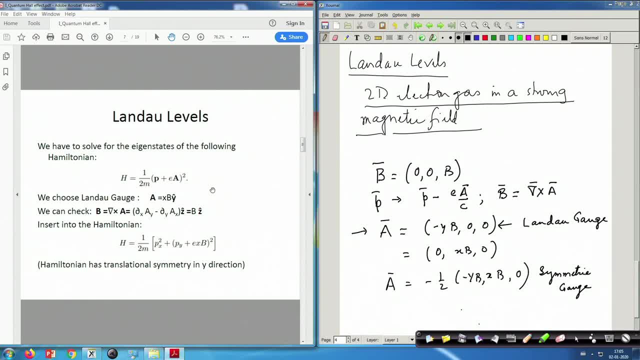 this one chooses this example, that the this view graph chooses the other gauge, that the y component is to be x times b. ok, But it does not matter, because the results do not depend on the choice of gauge. the final results will not depend on the choice of gauge. 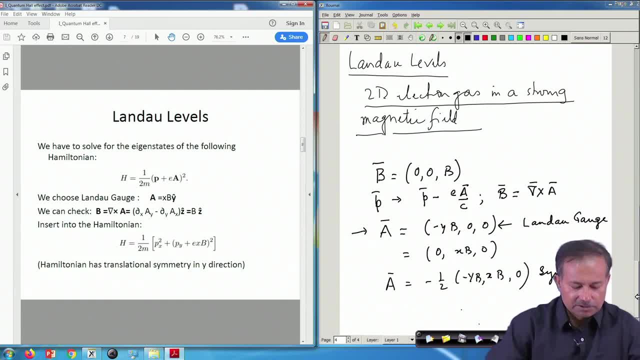 In fact the symmetric gauge is a is also a very popular choice. the algebra becomes interesting in that. So in: if you do this, then just replace. the way to do is: now is P. now the charge is negative. So P plus E, A by C for P you replace minus, i h cross. 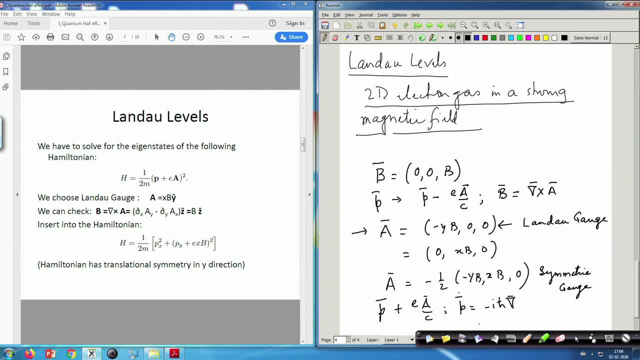 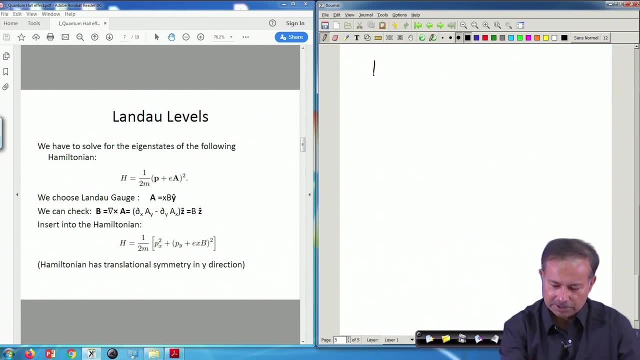 grad. So if you do that, then of course you will get back your Schrodinger equation. that is what the Schrodinger equation will look like now, So let me just write down the result that you will get in the gauge that I have just informed, h cross square by twice m into. 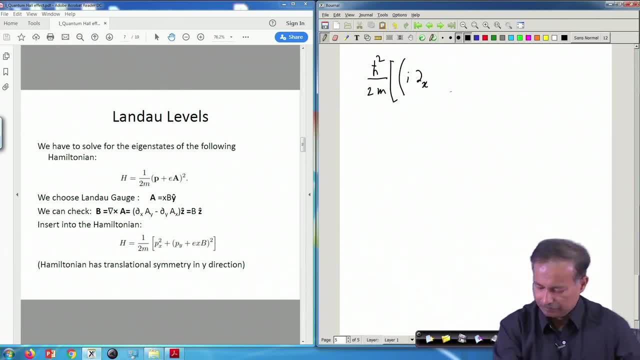 i del x. So that becomes your Schrodinger equation. Remember, this z component is just a free formula because it is a sorry. the z component is confined and in that direction you do not have a motion of the electron. So you are only concentrating on the x and y direction, and that is the way. 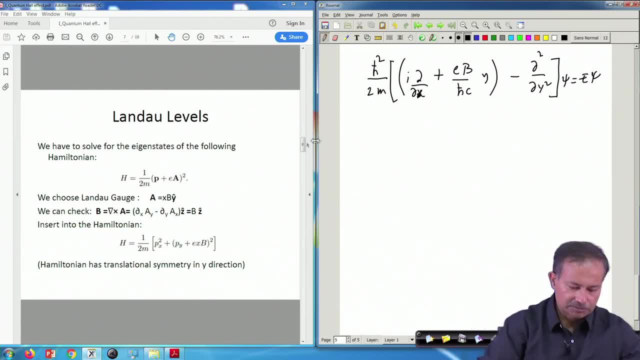 this thing is set up ok. So, for example, remember the Hamiltonian. still, as this says: in our case, the Hamiltonian has transition symmetry in the x direction. ok, 值 b to the power m to the power r. Sorry about it, It give i, k, x, some pi, times y. this is called the separation. 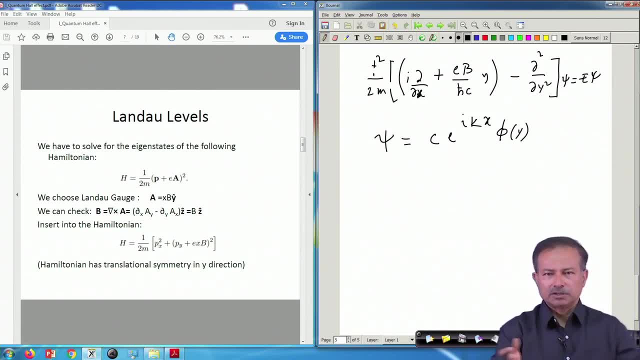 of variable. you have done it in hydrogen atom problems, done it in hydrogen atom problems or in many other cases. So what one does is that one chooses a plane wave, wave function along the x direction, because the transition symmetry exists in that direction still, And so one keeps that intact and write a plane wave state. 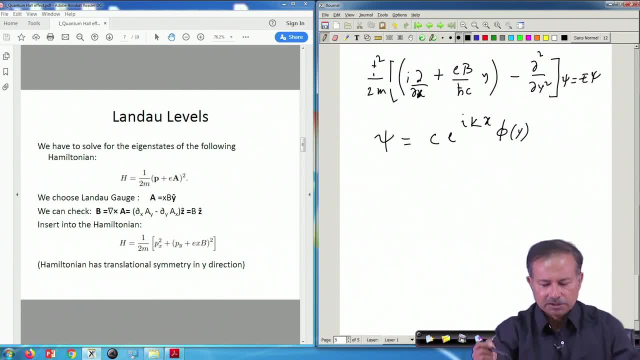 along the x direction, whereas in the y direction. of course you have to be careful because there is a term which you will change the nature of the wave function and what will happen, you will just see. So then you can just put this solution in. 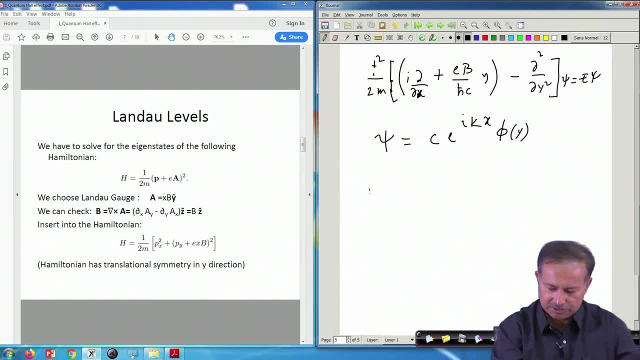 push. put this trial wave function in this and what you will land up is in is h cross omega c by 2.. Minus L, square del 2 del y, 2 plus y by L minus L k, this is that k square into phi y. 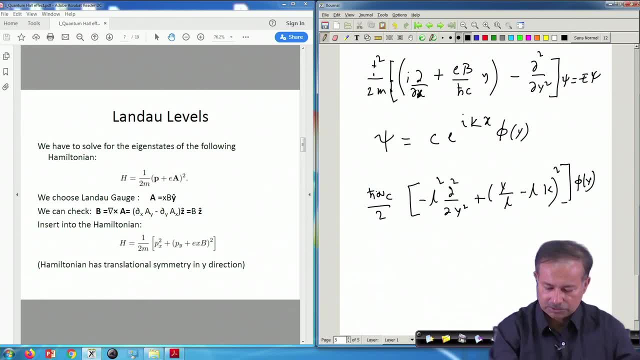 this is h cross omega c, equal to e phi y. So this is what you will get. where L is L square is h cross c by e v. So that is called. that is the magnetic length. this is all also written generally as L sub m to make it to: 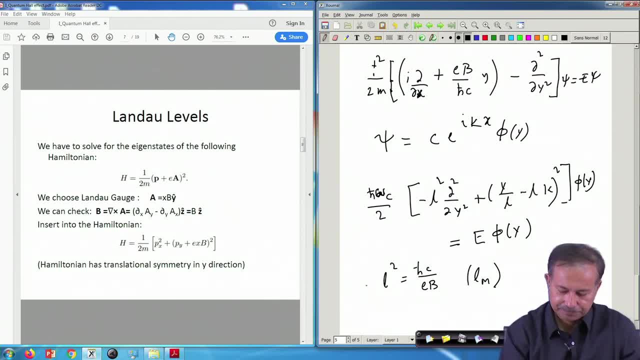 explicitly mention that there is. this is a magnetic length. Ok, It, as you can see that this h cross c and e are all fundamental constants and it is only inversely. L square is inversely proportional to B, So this defines a new length scale. 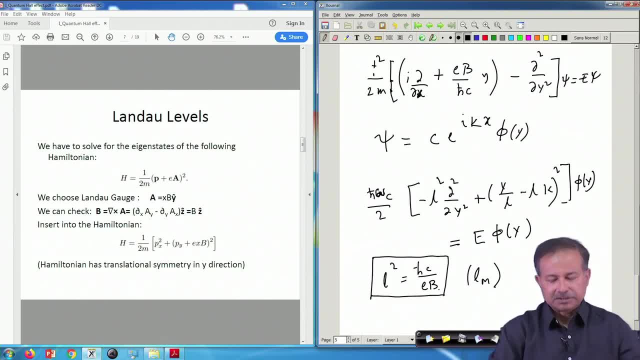 in the problem. It is interesting that from the algebra in a magnetic field- transverse magnetic field- a new length scale has now emerged in the problem and that length scale is dictated by the strength. By the strength of the field, the stronger the field, the. if you increase the field, the 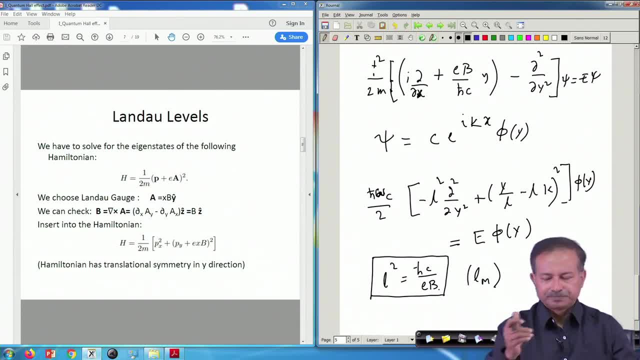 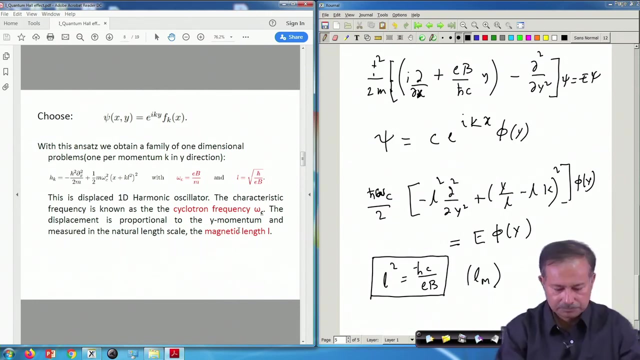 length scale decreases as a square root ok. 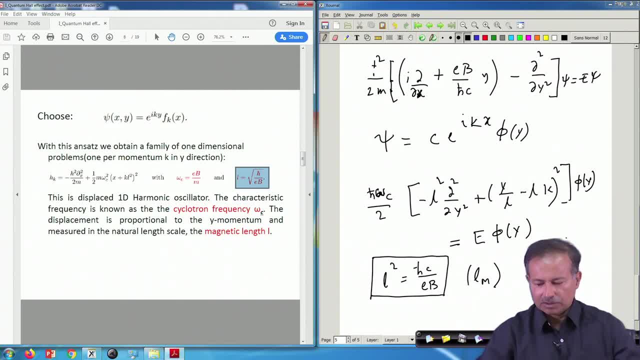 Now, if you look at this Hamiltonian that you got this equation: H psi equal to E psi. the left hand side represents a simple harmonic oscillator in one dimension. Suppose L, this k was 0, then this would be just a simple harmonic oscillator, right? 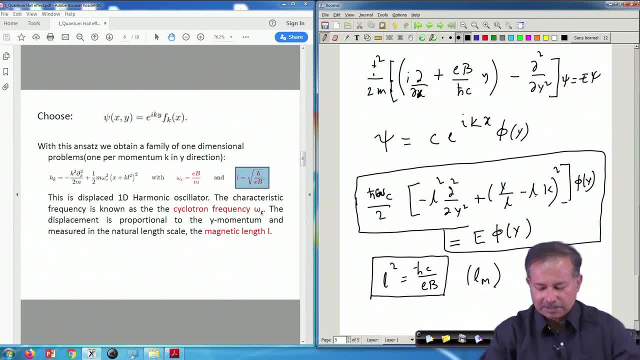 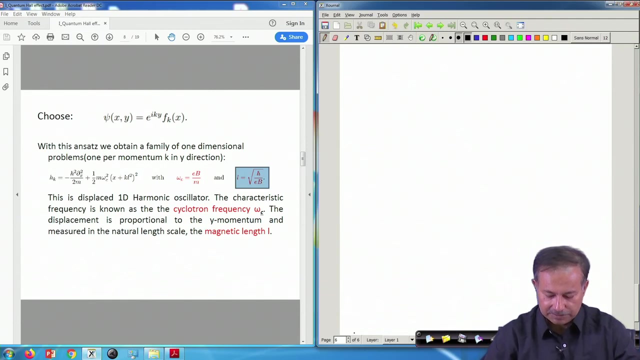 So that tells us that this problem has an interesting symmetry, that it becomes a simple harmonic oscillator problem in one direction and a plane wave in the other direction. So the solution then appears to be: can be written off, and remember that, because k- this term is nonzero- the, basically the center of that the oscillator has just been shifted. 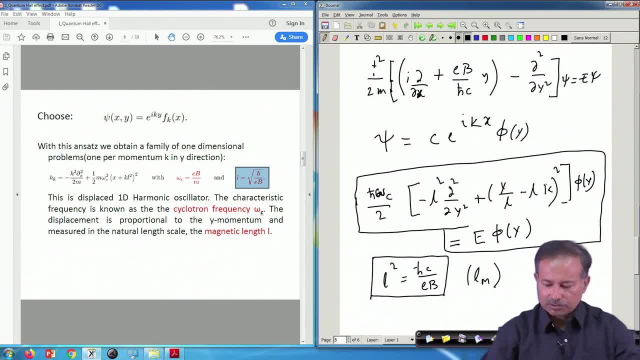 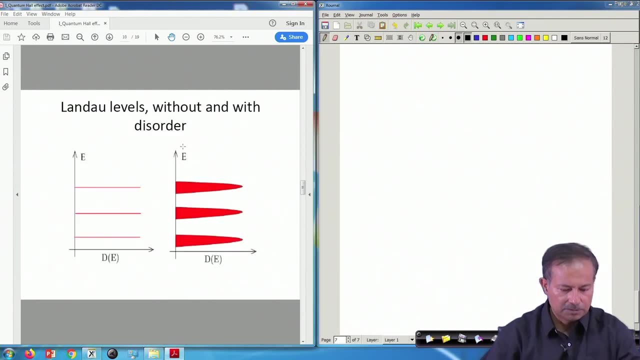 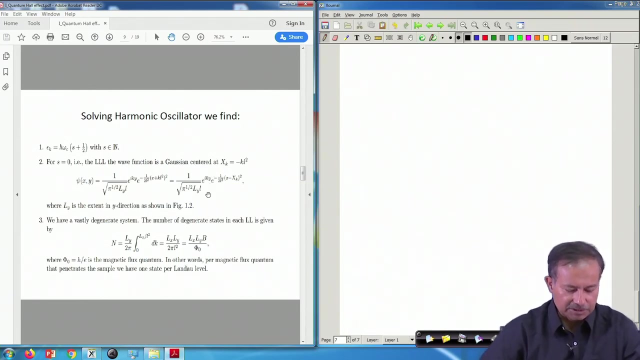 from y equal to 0.. So that is the amount of shift, L square k. So the center is away from 0 by amount L, L square k. So one can write down the solutions. and solution is basically a simple harmonic motion in one dimension, simple harmonic motion in y direction. 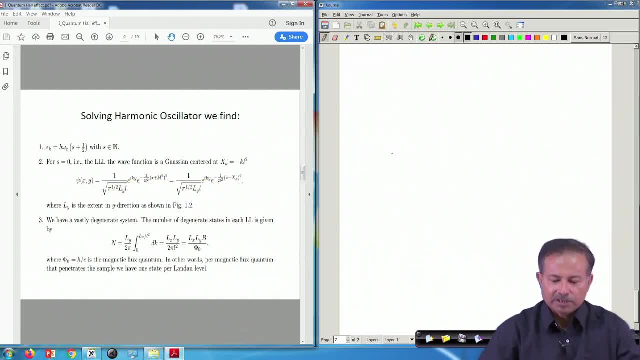 and a plane wave in the x direction. for my choice of gauge And for this one, for example, it is just the other way. it is a y. along y direction they have a. this has a plane wave and along the x direction it has a displaced harmonic oscillator. 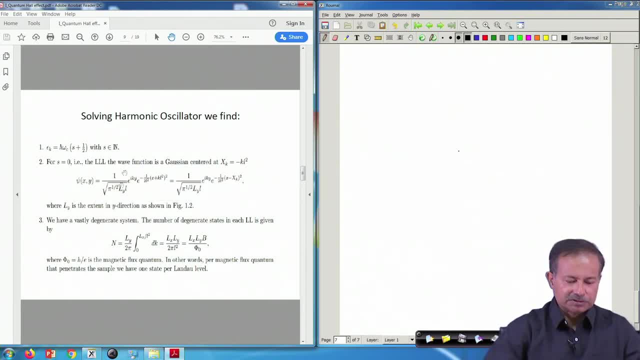 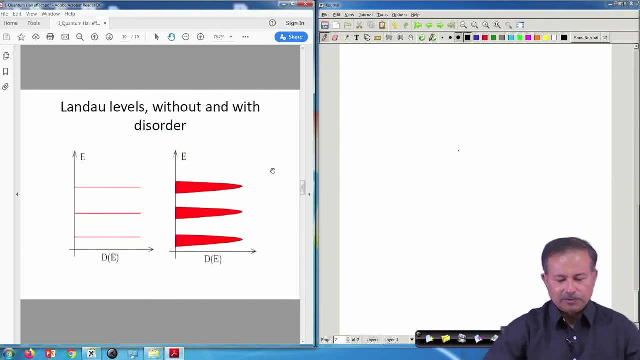 that is all. I purposely chose this example just to show you that two gauges do not differ in their final result. The solution remains the same, only the x and y gets interchanged with a minus sign, with sign plus to minus. as you have seen, the choice of gauge also involves a sign. Now, what does? 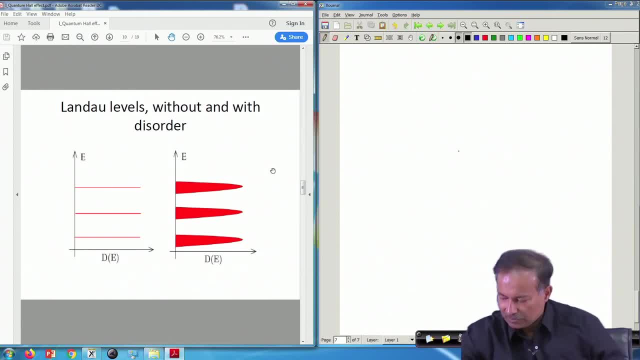 this lead to? Well, this leads to a So wave function of the form phi, phi, n k plus n. what this n is, I will tell you. equal to some constant, some, this is a Hermite polynomial. remember your simple harmonic motion: y by L minus L, k, e to the power exponential minus. 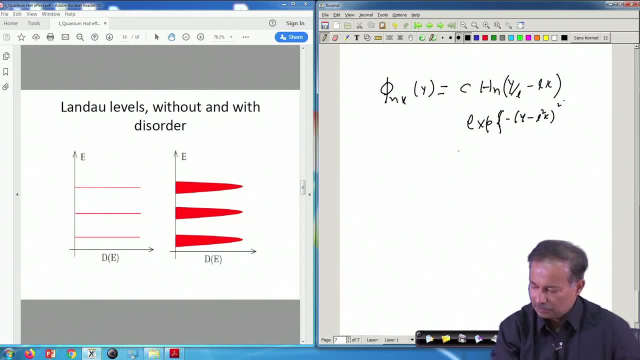 y minus L square k square. Ok, By twice L square. So this is the one can write it as e to the power. then you can see the similarity clearly, that this is a e to the power minus y, minus L square k. So we: 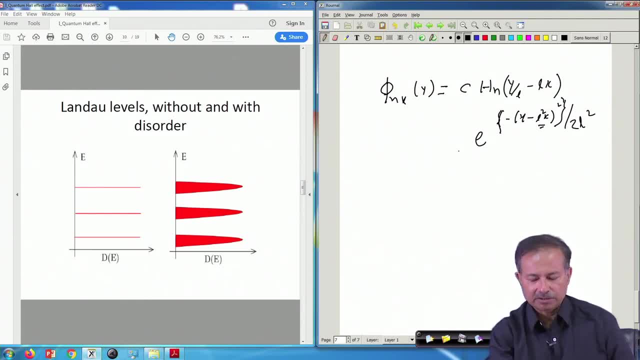 had this part not been there, this would just be e to the power minus y square by 2 L square, which is a simple harmonic oscillator with origin at 0.. Now you have the origin shifted by an amount: L square k. So that is the solution and 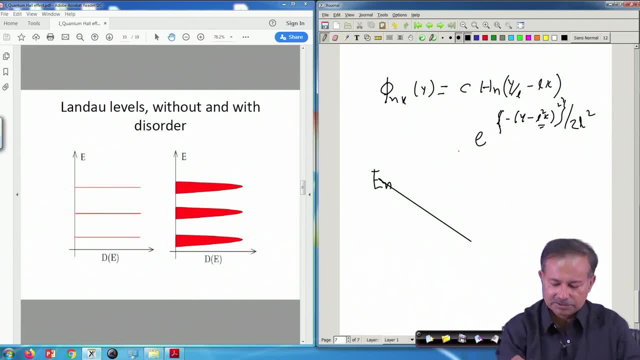 the energy this n comes from. this, sorry about it- is n k, n. k is actually independent of k. h cross 3 into k. So if this is true, that means then E square 1 is in this form, in w k. this is what, And this is a very simple f25 k. So I am giving argument for this. Due to this, we are curves- and this is a very simple argument- where this, which is to the power exponential minus E square k, into L square, k square. now, if you come to this, may on this Screw. 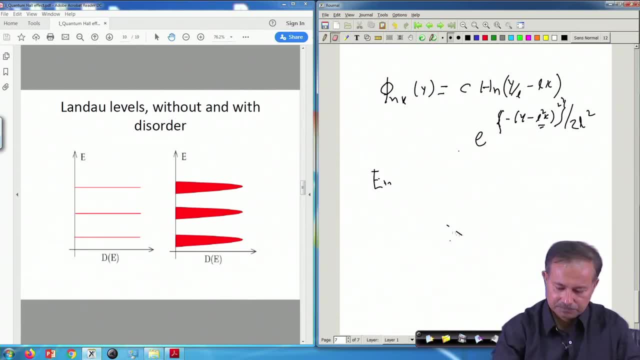 k is actually independent of k. h cross n plus half and this n is an integer. omega c, as before, is E b by m c, So h cross omega c is the scale of energy. I mean this is exactly like a harmonic oscillator, So the harmonic it is like. there is this: 0 point energy at n. 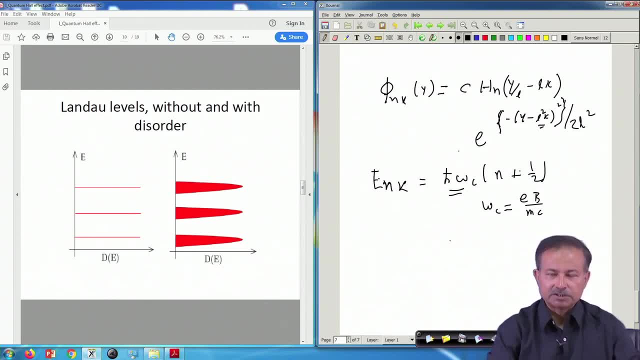 equal to 0, you will still have a finite energy, as happens in any confined potential, for example, and the oscillator potential is a confining potential, And h cross omega c into n plus half, So that has the has. the same is the same form that you get from the lander, from the 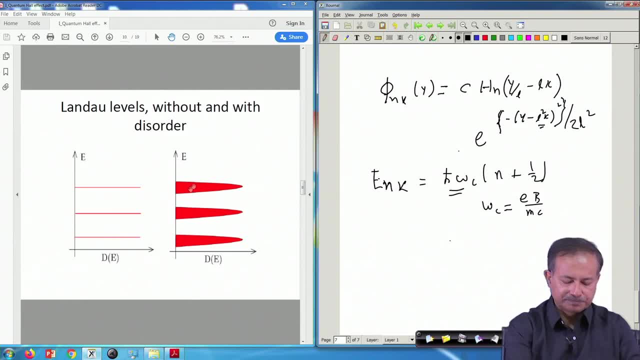 oscillator, So that. so that means that the energies are quantized in this form, that energy at. as a function of this is density of states written. but if you write the other way, which is so, let me just draw it the way we normally draw. E is, E is basically a series of lines. 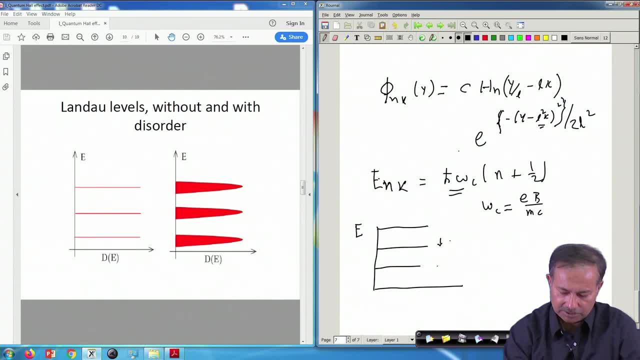 which is, which are separated by an amount: h cross omega c, And there the separation is constant. So here you can see that the studying goes on and on. now this x axis. let me just keep it for the time being. but this is the, just the energy. look at the energy and this is: 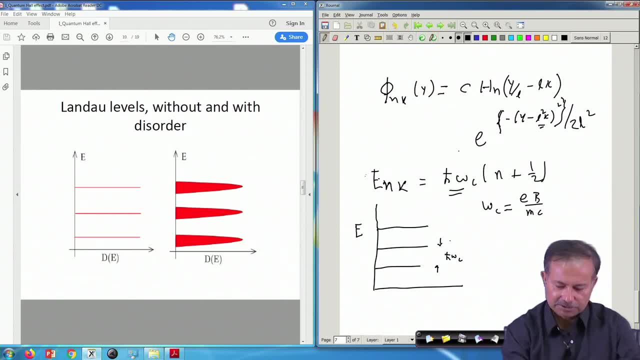 how it pans out. the result tells you that this is how it this discreteness of the energy as just like a harmonic oscillator. The interesting thing is that this is the way. if you just divide this by h, cross omega c, then these will be 1,, 2,, 3,, 4 and so on. Now, if you have b equal to 0, then of course, 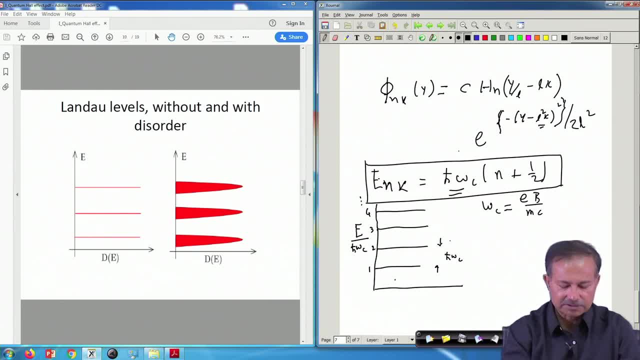 this will not happen. this will be just the two dimensional case where we know that the two dimension free particle case, right, with the density of states, which is constant. ok, So this plot on the left, for example, gives you the density of states as a function of: